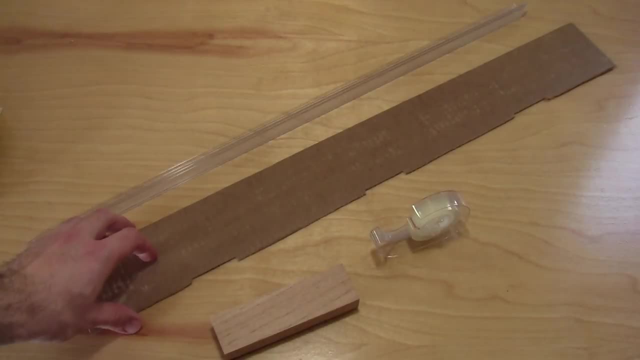 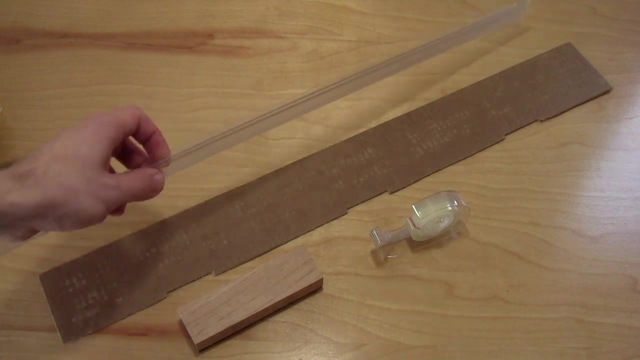 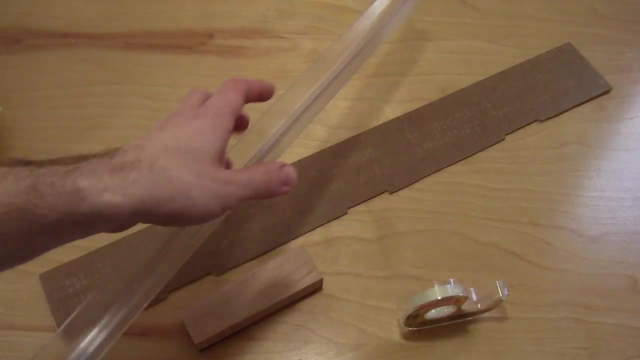 will lose their stickiness. Next, cut off one of the long sides of the cardboard box, Take your wooden block of the train and the two plastic angle pieces from your kit and clear double-sided tape which you need to supply separately. Your goal will be to attach. 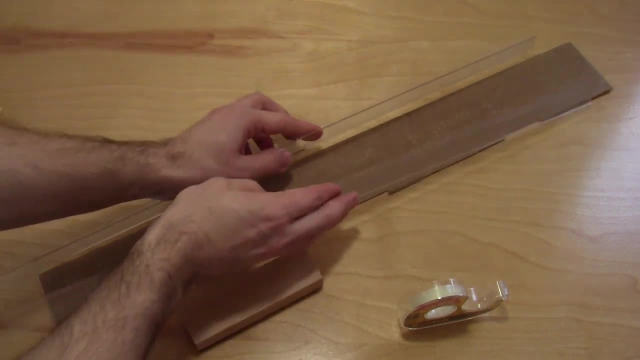 the plastic angle pieces so they are facing up. Then you will need to cut off one of the two side pieces of the cardboard box and then glue them together- Make sure you line them up straight- and then cut off one of the two side pieces of the cardboard box. 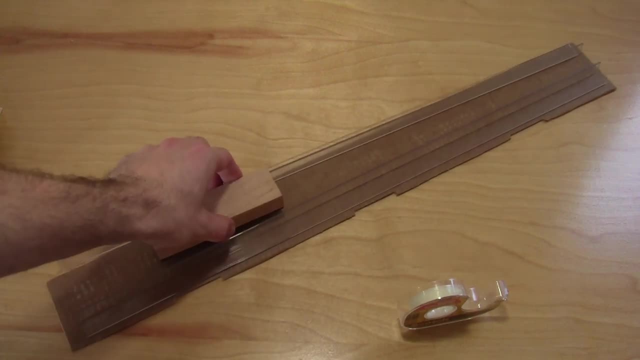 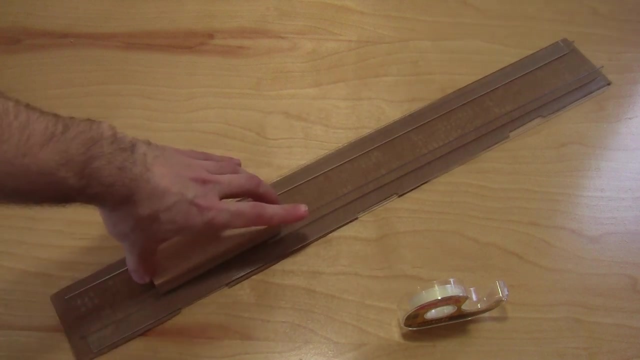 Now you can take your wooden block and use it as a spacer in between the angles. Move them out a little bit more, so there's about a millimeter of space. This will make sure that the train can slide back and forth without getting stuck between the angles. 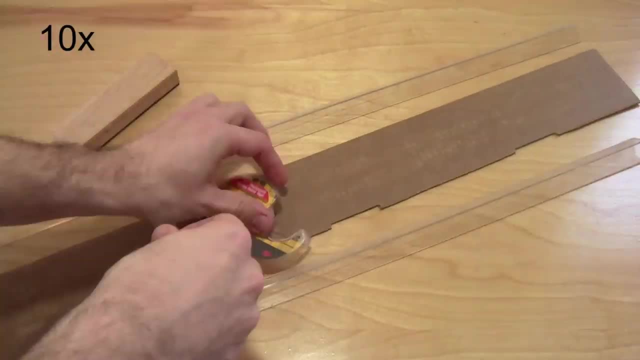 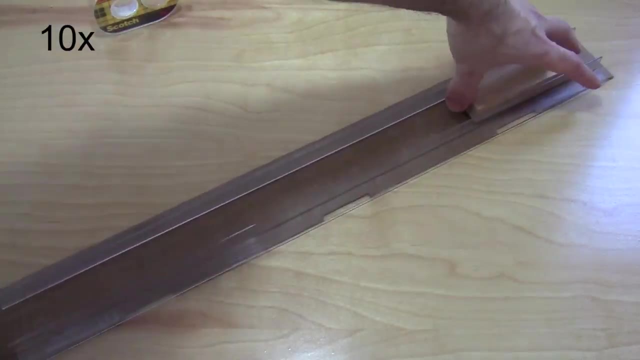 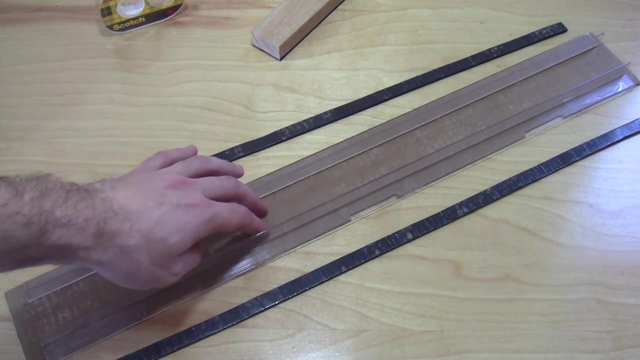 You can use the spacer to make sure the train can slide back and forth without getting stuck between the angles. Next, take the two long magnetic strips from the kit and you're going to attach these parallel to each other in between the plastic angles. You'll want these strips to be slightly closer together than the strips on the bottom of. 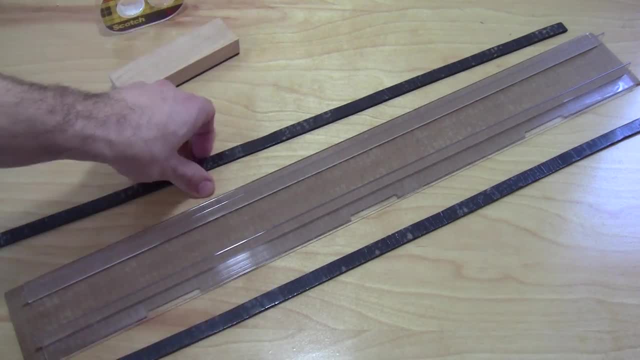 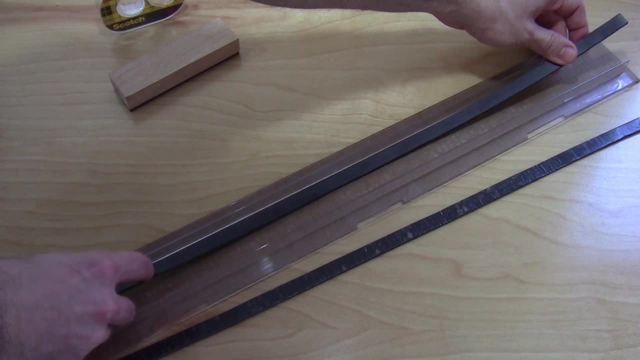 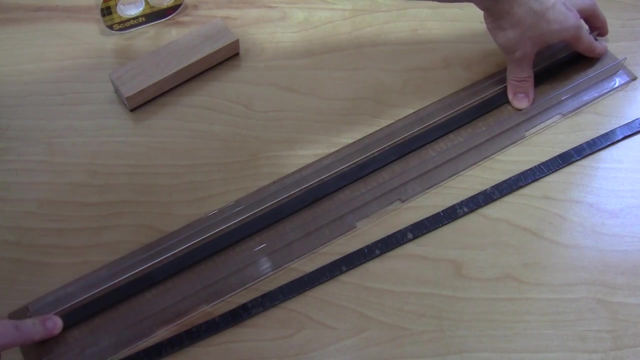 your train, as this will help the train balance. Now these are a little harder to apply because they're long and rather flexible. So put one down first a couple millimeters in from the plastic angle and again, if you mess up, you can peel these off and reattach them. just try not to do that too many times. 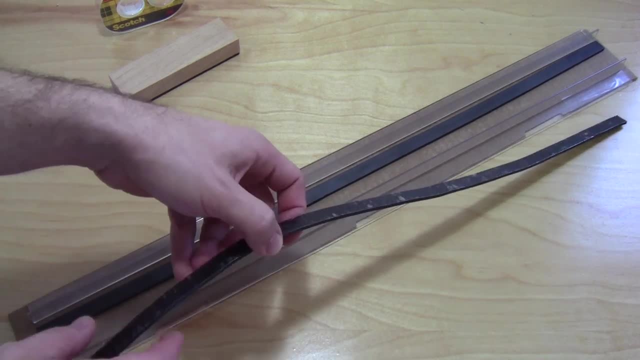 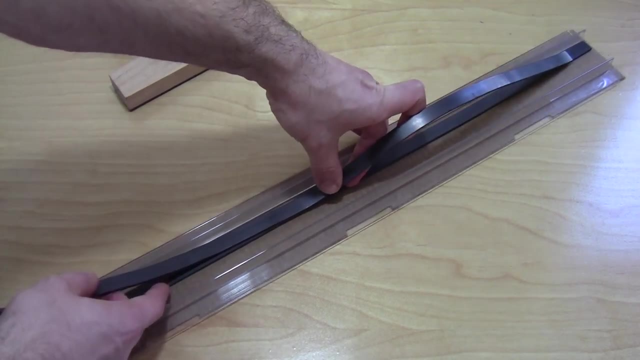 as they will gradually lose their stickiness. But you could also use clear double-sided tape if the built-in tape starts to lose its stickiness too much. Now there's something to watch out for: The strips will try to attract to each other, since they're long and flexible, so you have 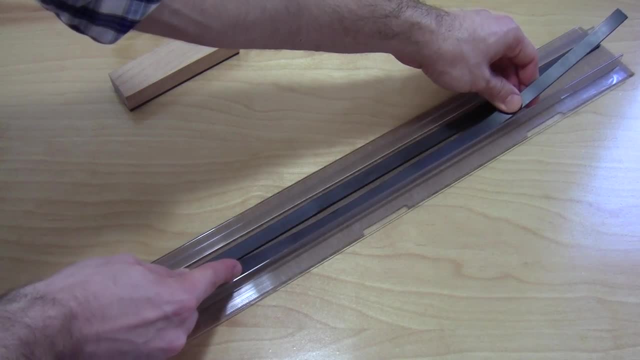 to hold the second one off to the side, as you put it in, And then, once you have them in place, you're going to want to pull them out of the way. And then, once you have them in place, you're going to want to pull them out of the way. 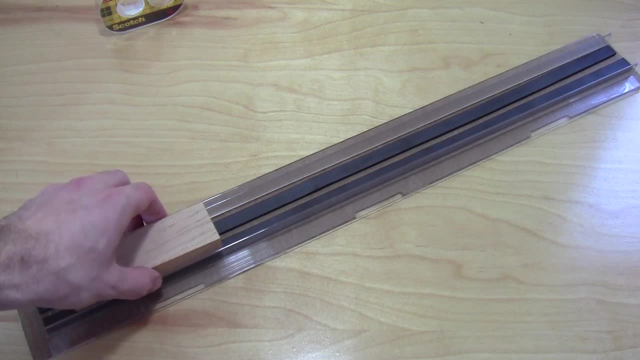 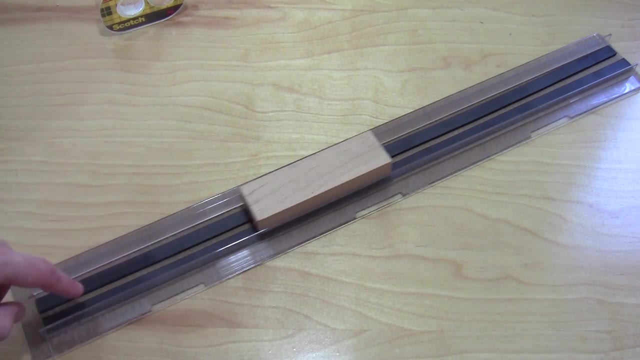 Once you have both strips pressed down, test your train. Put the train in between the angles and it should be able to slide back and forth easily without getting stuck. A good way to test is just to give the train a flick with your finger and it should glide.